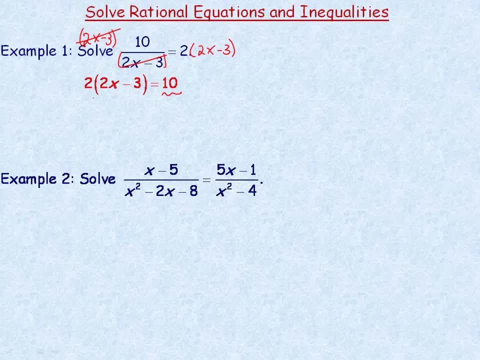 doesn't matter whether the 10 is written on the right or the left side, or the 2 times 2x minus 3, you can write them on either side there. Now, some people will actually do this also. this is just a little slightly. 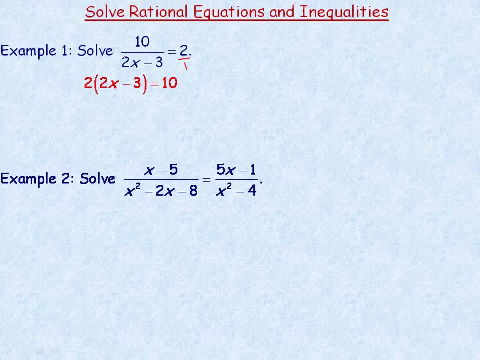 different procedure. right, the 2 is 2 over 1, so if I'm cross multiplying 2 times 2x minus 3, that product would equal the product of the 10 and the 1, which of course is the 10 on the right side here. So either way we end up with 2. 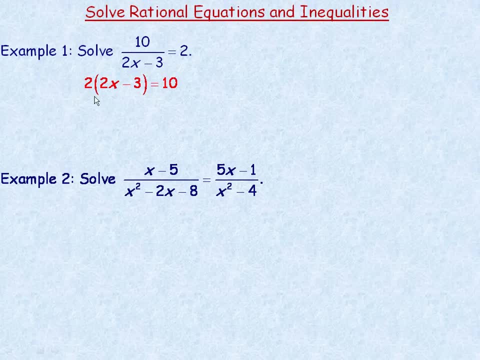 times 2x minus 3 equals 10.. Now what I would do next is expand out this left side. so 2 times 2x minus 3 is 4x minus 6.. Don't forget to multiply the 2 by that 3, and. 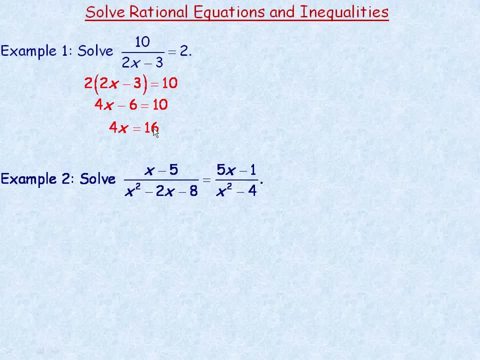 I'll add 6 to both sides. so now I have 4x equals 16, and then dividing out the 4,: 16 divided by 4 is 4, so x equals 4.. Now in example 2, I have two different denominator. 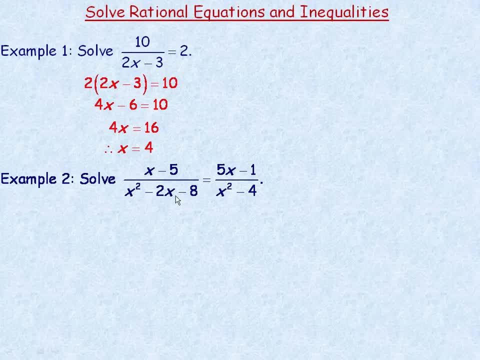 expressions here and while they won't always factor and common factors divide out, you should always should try that. It will make your simpler. So I'm going to factor both the denominators. On the left, here the denominator, we have a minus 2x and a minus 8, so look for numbers that add to. 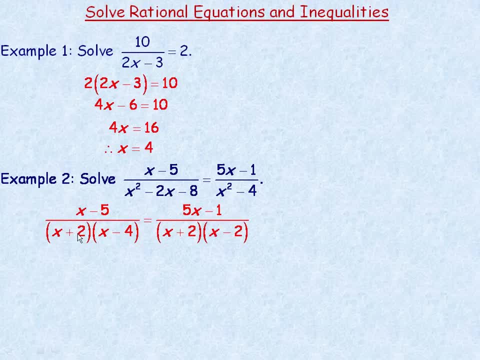 negative 2 and multiply to negative 8, and those two numbers are positive 2 and negative 4.. And so this x squared minus 2x minus 8 would factor into x plus 2 and x minus 4.. x squared minus 4,, that's the difference of two perfect squares. so 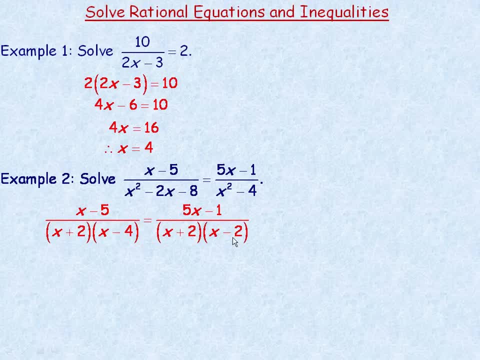 that'll factor into x plus 2 times x minus 2.. And so once again, notice- we're going to multiply both sides by notice that there's an x plus 2 factor in both denominators, And so those x plus 2s will divide out and the reason they'll. 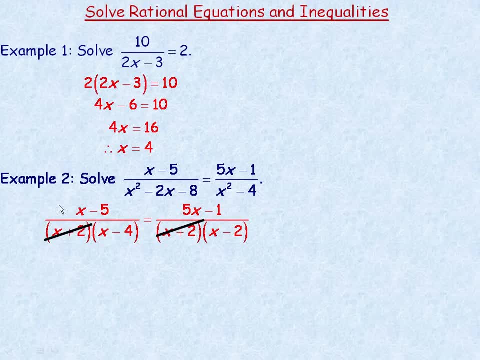 divide out is because if I multiply both sides by x plus 2- now like let's pretend they were 2, and I multiply both sides by x plus 2, and I multiply both sides by x plus 2, they're not divided out yet Like this x plus 2.. Then actually what? 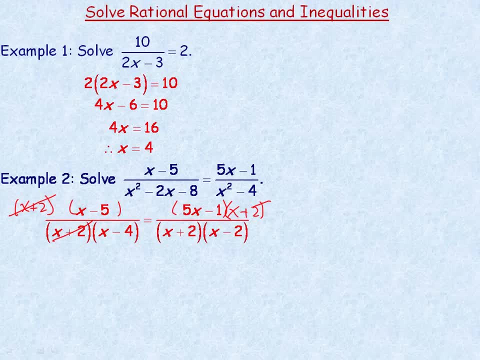 happens is that x plus 2 divides out with that one and this x plus 2 on the right divides out with this one. Okay, so we would just then have left the x minus 5 over x minus 4 on the left equals 5x minus 1 over x minus 2 on the right. So 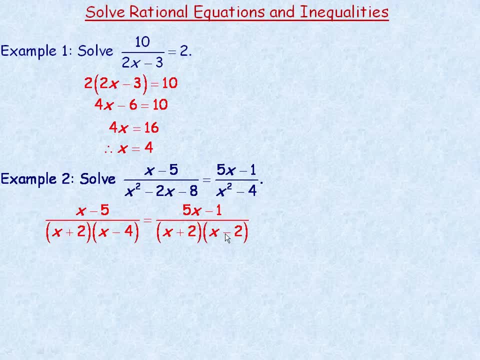 we go back to this, so the x plus 2s are divided out. Now there's still an x minus 4 here and an x minus 2 here. So again, like I did in the example above, I would still want to rearrange it. so there's no rational expressions. So I'm going to 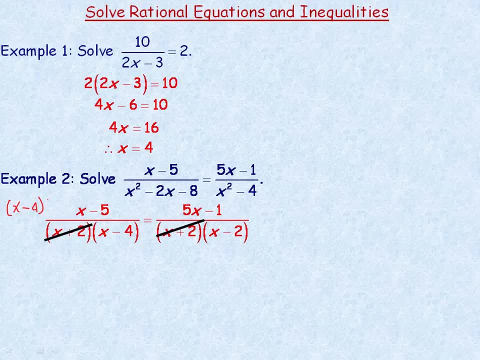 multiply now by x minus 4 times x minus 2.. Notice, that's the two factors in the denominators, One on each side. So x minus 4, x minus 2.. So on the left here this x minus 4. 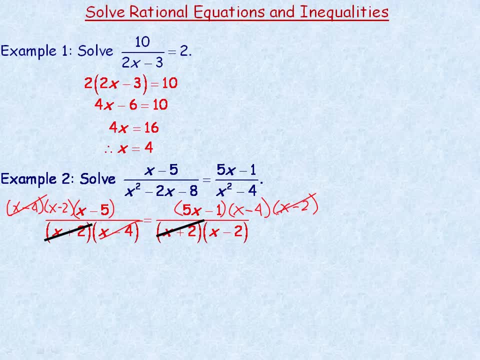 divides into that one, and on the right side, this x minus 2 divides into that one. So what I'm left with now is 5x minus 1 times x minus 4, multiplied is equal to the product of x minus 2 and x minus 5.. It really doesn't matter that. 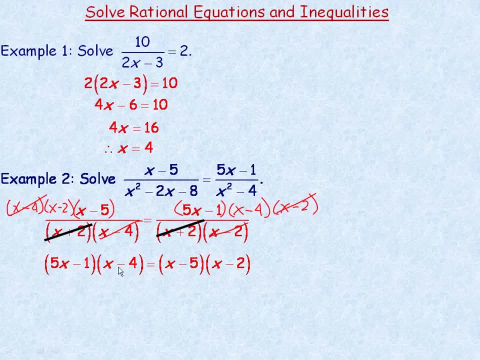 that was on the right and this is on the left. now it doesn't matter at all. You could do that by multiplying both sides by x minus 4, and on the right side you can write them on either side, And so I'll now expand out each of the 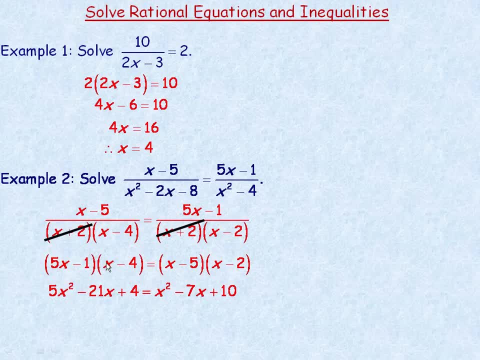 sides here: 5x minus 1 times x minus 4.. 5x times x is 5x squared. 5x times negative 4, that's negative 20x and this would be a negative 1x and they add to negative. 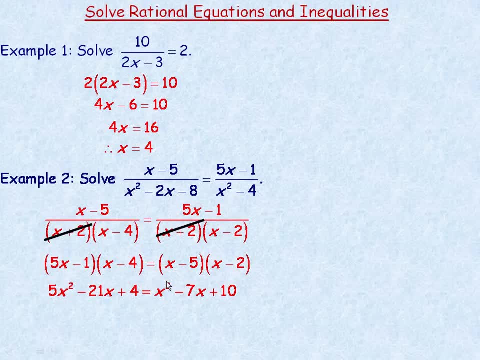 21x And negative 1 times negative. 4 is 4.. On the right side, x times x is x squared: x times negative. 2 would be negative 2x. We have negative 2x and this would be negative 5x. 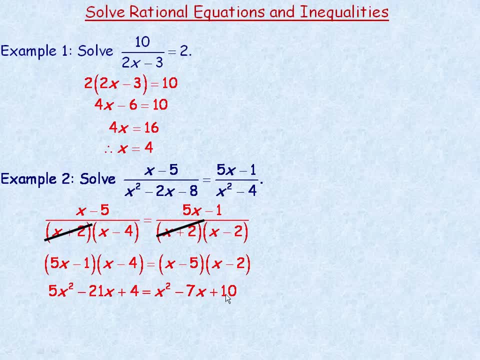 to give us negative 7x And negative 5 times negative. 2 is positive 10.. So now I would rearrange and set everything on one side equal to 0.. So subtracting x squared from both sides, 5x squared minus 1x squared is 4x squared, Adding 7x. 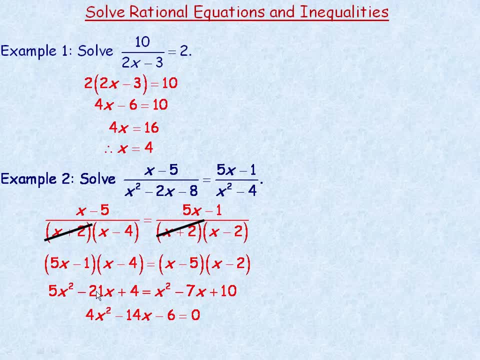 to both sides, because I want a 0 on the right side here. adding 7x to both sides- negative 21x plus 7x is negative 14x, And then subtracting 10 from both sides, 4 minus 10- is negative 6.. 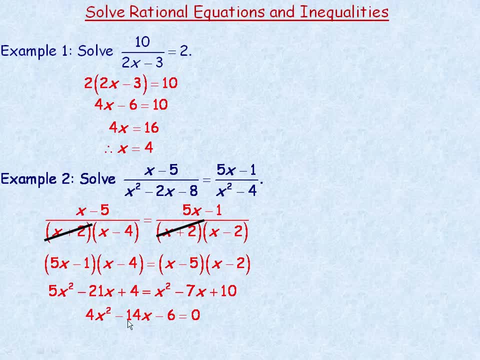 Now we could try to factor this, but this actually doesn't factor. There are no numbers that add to negative 14 and multiply to negative 24.. So I still may be able to solve this. And to make it a little simpler to solve, we can actually divide. 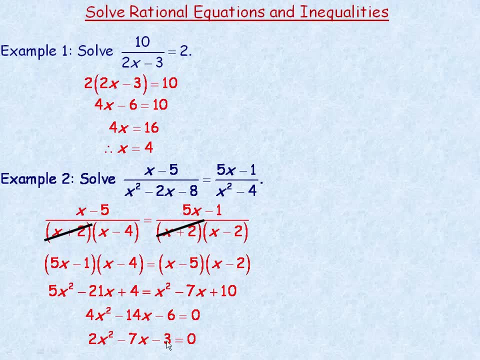 everything by 2, but there still are no numbers that add to negative 7 and multiply to negative 6.. They don't exist, So we would bring in the quadratic formula, And so a is 2,, b is negative 7, and the constant c is negative. 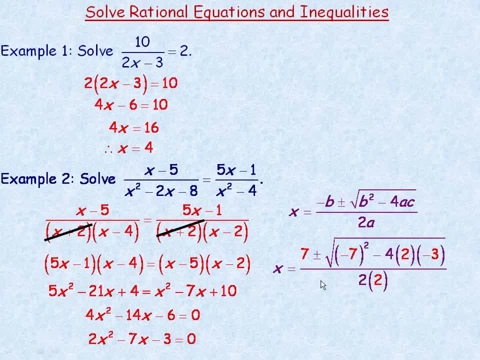 3.. So substituting those in our formula we get this. So underneath the root sign this would be 49.. And notice, we have minus 4 times and there's also a negative 3 here. so we'll be adding 4 times 2 times 3.. So 4 times 2 is 8, times 3 is 24.. So 49. 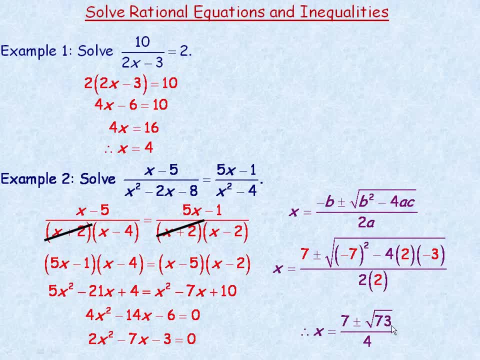 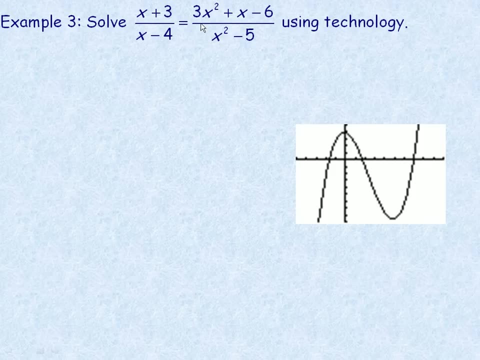 plus 24 underneath the radical adds to 73. So we have the solutions are 7 plus or minus the root of 73 over 4.. Of course in the denominator 2 times 2 is the 4.. In the last rational equations example we have this expression here and once. 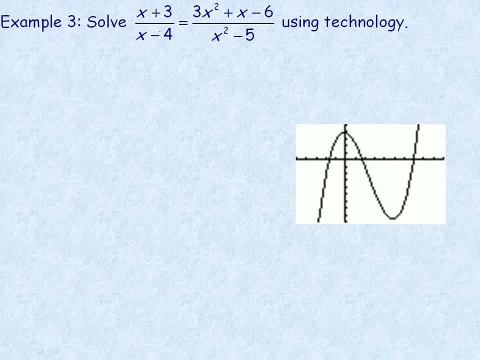 again, I want to get rid of the rational expressions And I will do that by now. x squared minus 5 and x minus 4 do not factor. Okay, so we're not going to be able to divide out any common factors. So the two factors are x minus 4 and the x. 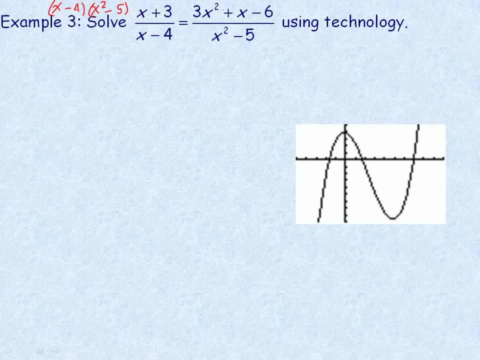 squared minus 4.. Minus 5.. So we'll multiply both sides by the product of those two factors. And so, on the left, this x minus 4 divides into that one, and on the right side, this x squared minus 5 divides over that x squared minus 5.. And so what we're left? 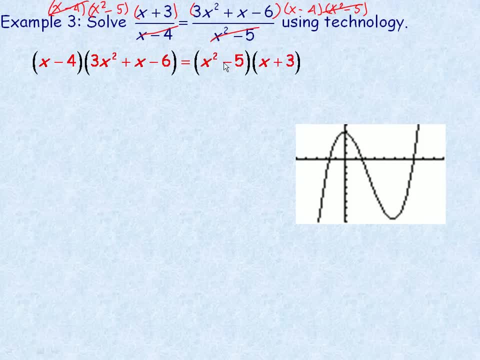 with, then is x squared minus 5 times x plus 3, that product is equal to the product of x minus 4.. And 3x squared plus x minus 6.. And so now, the goal now will be to expand out.